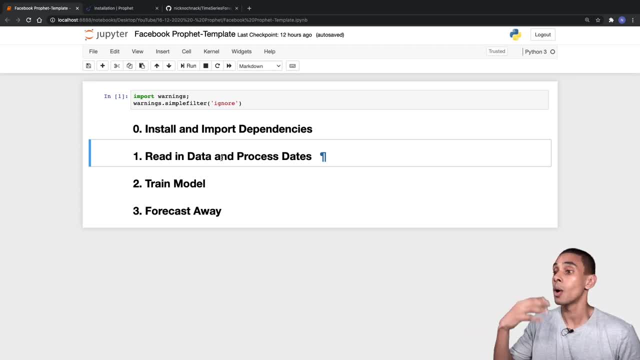 you could definitely just sub in the model here, And I'll actually comment as to when you can do that. So, basically, you're just going to do this, So you're going to do this, So you're going to just going to be shifting your data set and plugging in your own rather than using the one. 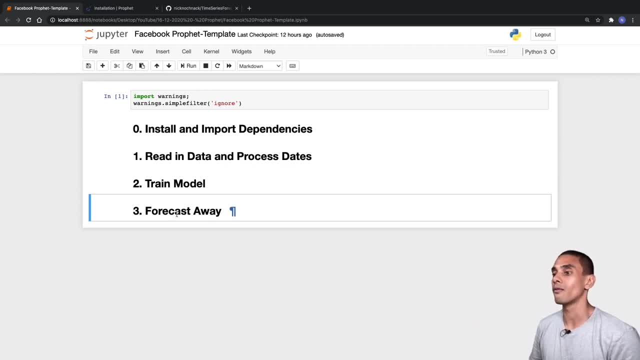 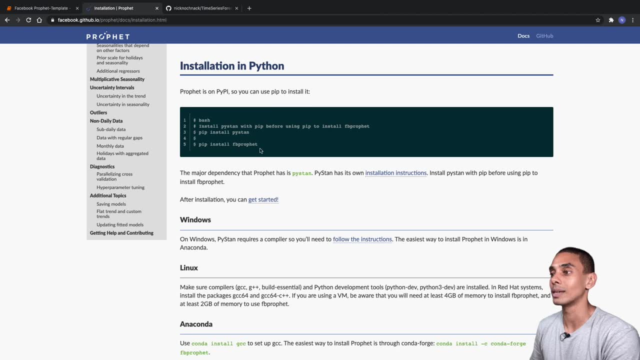 that I've provided, Then what we're going to do is train our model and then forecast away. So in order to do this, we're obviously going to be needing a Facebook profit. So in order to install it, we really just need to run these two commands here. So pip install, PyStand and pip install. 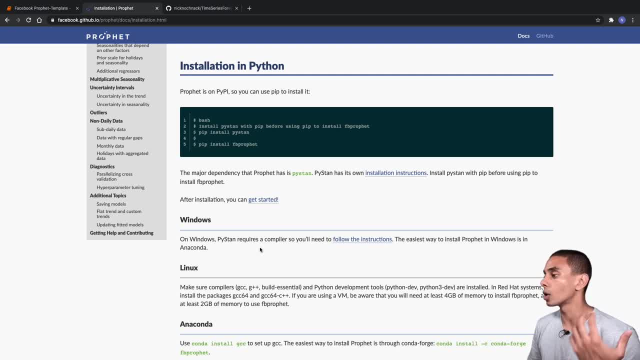 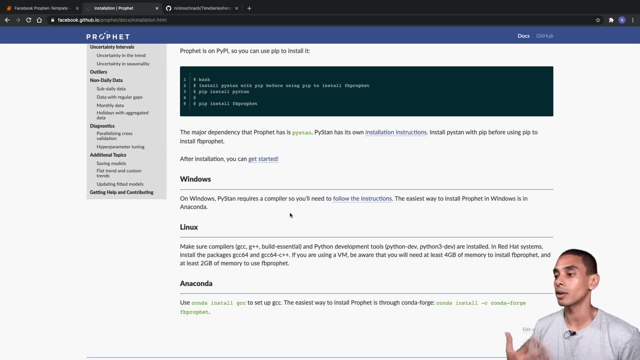 Facebook profit. Now, if you are running on Windows, you're going to need a compiler, So I'll include a link to this in terms of how to go ahead and install that. If you're running on a Mac or a Linux machine, it's a little bit more simple. Now, also, if you want the code for this, 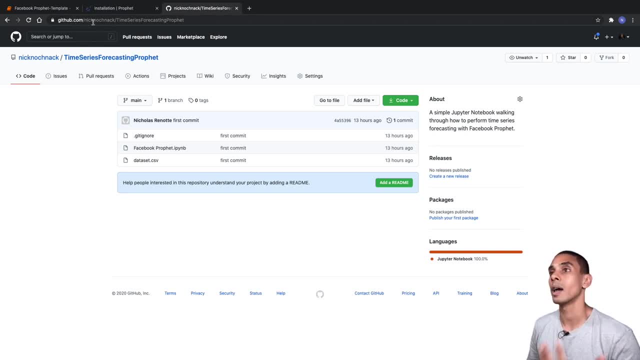 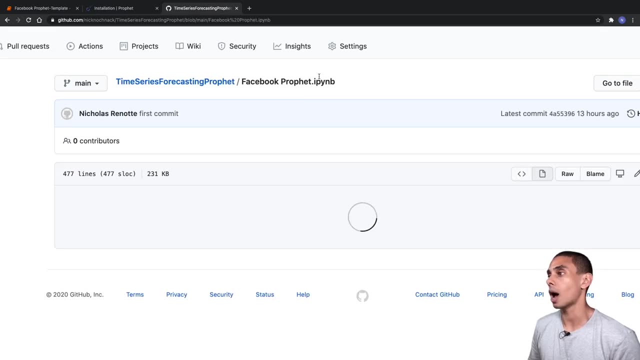 tutorial: just go to githubcom. forward slash, nicknockknack, forward slash- time series- forecasting profit, And I've included the Jupyter Notebook, So it's called facebookprofitipynb, which includes all the code that we're going to write, as well as a test data set, So you can see it's all written. 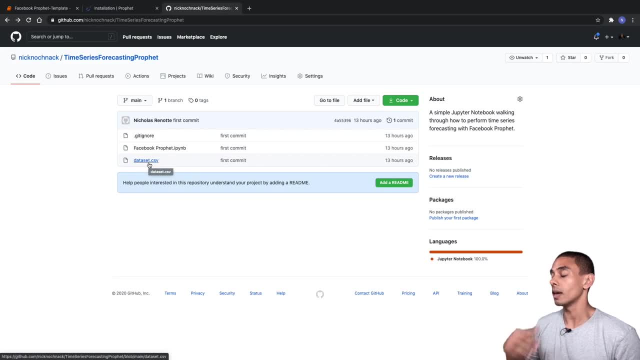 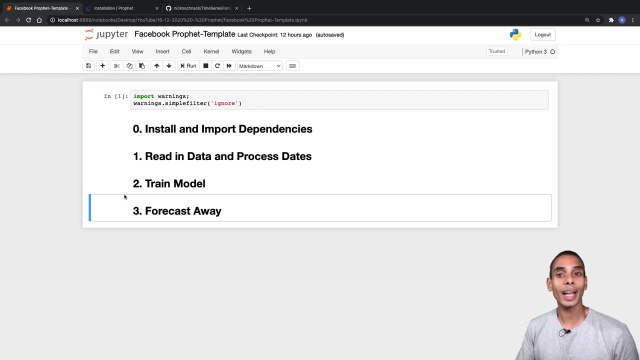 there And we've also got a data set, so datasetcsv. So if you want to pick this up, really easy, So just go and clone down this repo and you'll be able to run this. So if you want to through it Now, in this case we're going to do it from scratch and explain each one of the 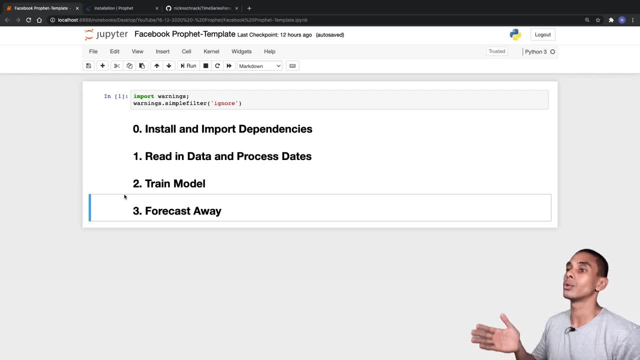 different components involved. So, first up, what we need to do is install and import our dependencies. So, as I said, we need PyStand and we need profit. Now I've already got pandas installed, so I don't need to install that. But if you don't, then make sure you include that as 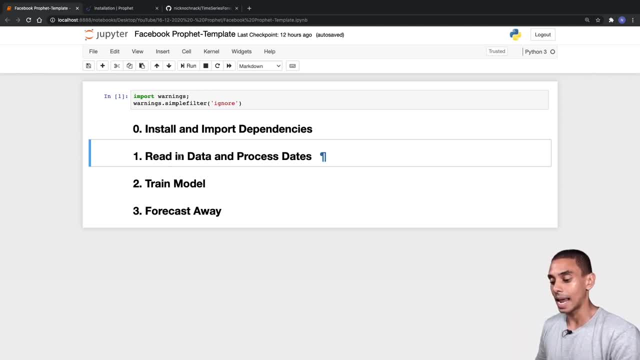 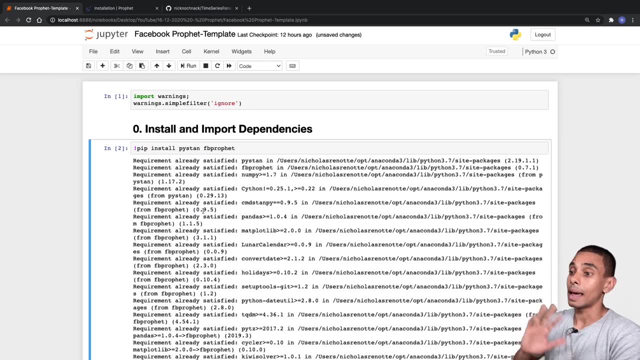 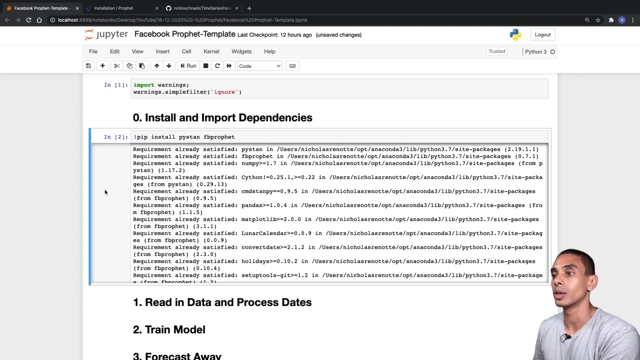 part of your pip install command. So first up, let's go ahead and install PyStand and profit. I already had it installed so it went pretty quickly. If you're installing it for the first time it might take a little bit longer. So in terms of the command that we ran, it's exclamation: 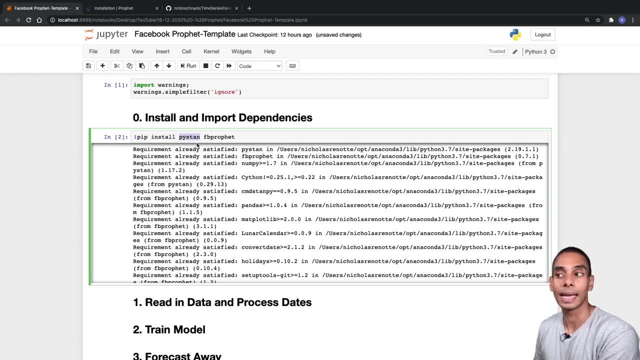 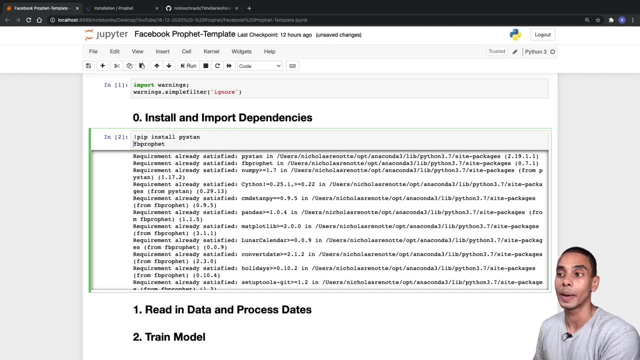 mark pip, install PyStand, so P-Y-S-T-A-N, and then space FB profit. So this basically allows us to install both packages on a single line. Normally what I'll do is I'll space it out on two different lines. So you can see that. but in this case pretty straightforward: pip, install PyStand and 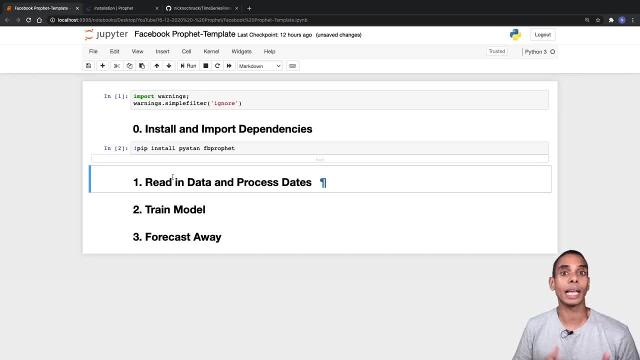 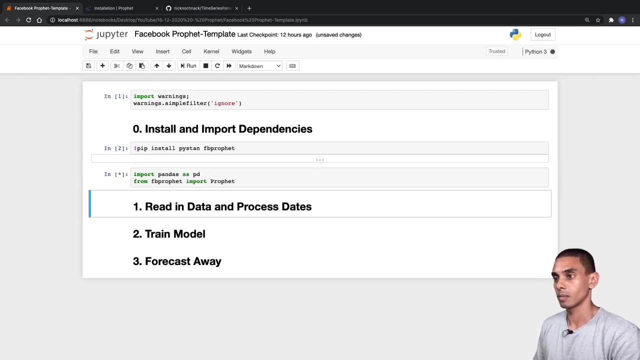 Facebook profit and you're good to go. Now the next thing that we need to do is actually import pandas, So let's go ahead and import them, Alrighty? so we've now gone and imported our dependencies, So you can see that we've imported pandas And in order to do that, I've written. 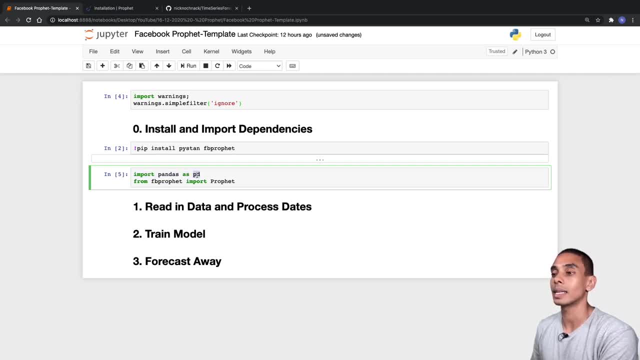 import pandas as PD. So this basically allows us to take the pandas library and just shorten it so that we can just call it by using PD, Then from Facebook profit. so we've run from FB profit and then from Facebook profit. we've run from FB profit and then from Facebook profit and then from. 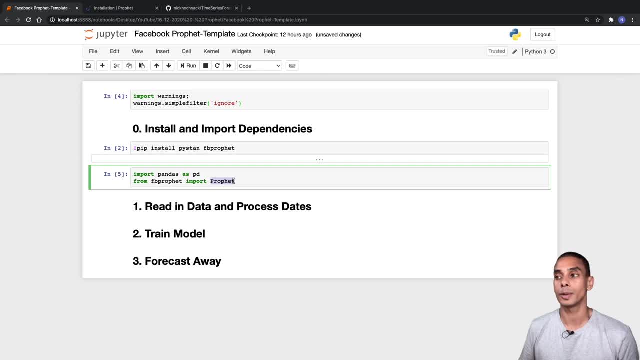 Facebook profit, import profit, So this gives us all of our profit dependencies. Another quick thing to call out that I forgot to mention, So I've just imported warnings and ignored any of the simple warnings. So basically, whenever you're working in profit, you get these big red warnings. 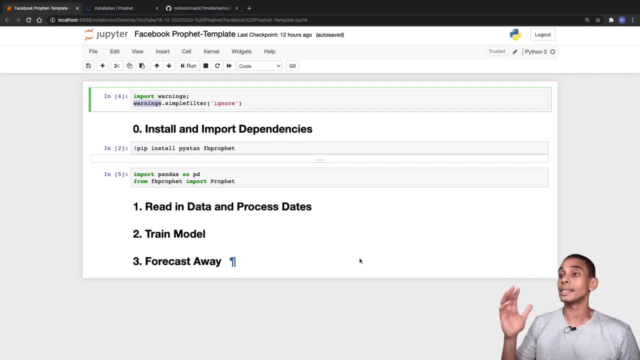 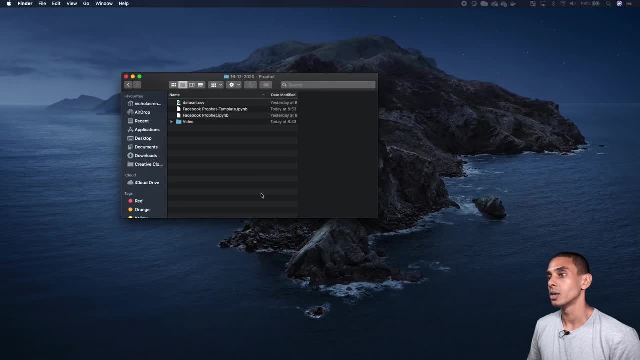 sometimes, So this just makes it a little bit cleaner. All right, so that's our dependency: installed and imported. Now what we need to do is read in some data and process our dates. So in this particular case, we're going to be working with this data set here, So it's called datasetcs5.. 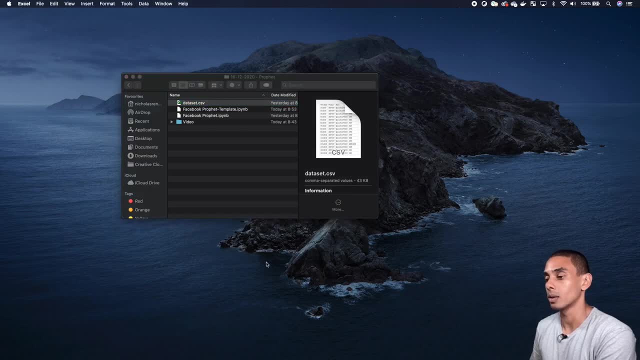 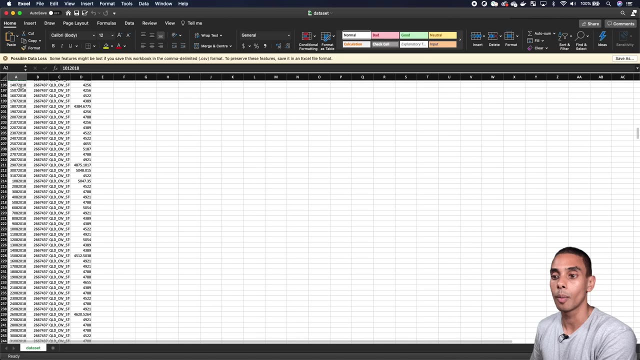 Now, if we open this up, let's take a look at what it looks like. So you can see that we've got a column with a time date and this includes a whole bunch of dates, and it looks like it goes until about end of 2020.. And then we've also got two other columns for 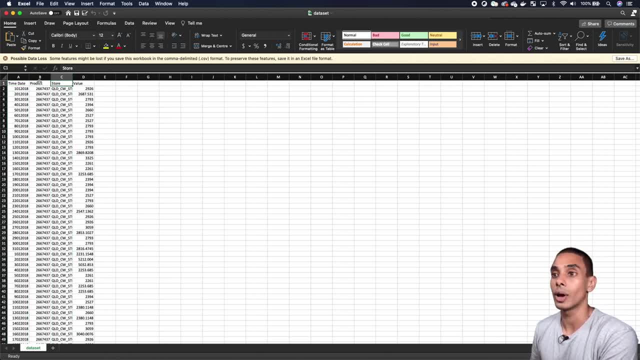 product and store. So these look like they might be product and store related, to add to that level. So when we're performing our summary statistics within pandas, we just want to make sure that we've only got a single product and a single store, because we're predicting one single time series. 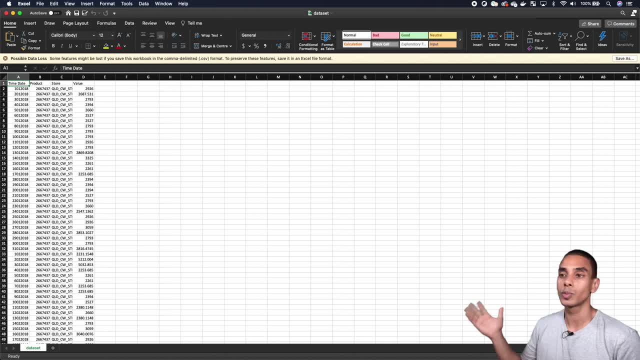 Now, if you wanted to, you could loop through and produce multiple sets of time series forecast. In this case, we're just going to be doing one, So it looks like we've also got a value column as well. All righty, back to our Jupyter Notebook. So now what we're going to do is read it in. So 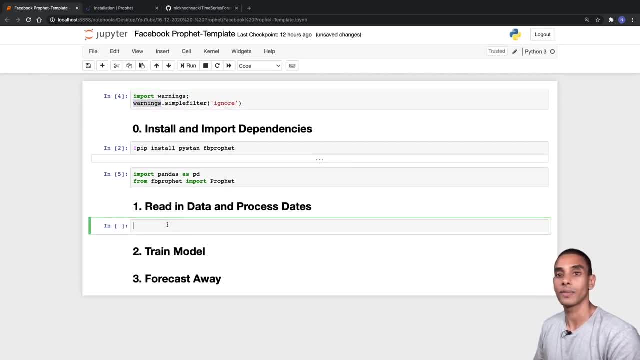 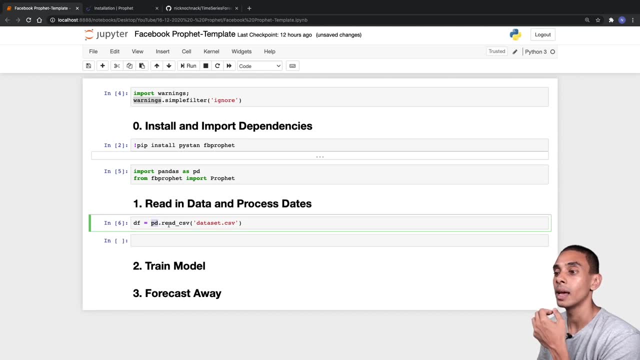 in order to read in our data set. we're going to use the read CSV method, So let's do it, All righty. so we've written df equals pd, dot- read CSV. So this is a pandas method. So you can see that we've got our shortened form of pandas over here. 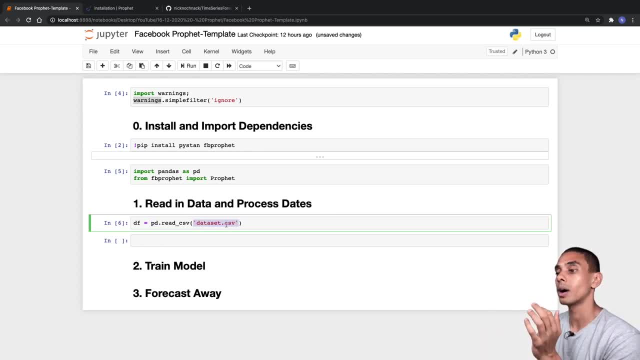 And then we've passed through the name and the full path to our data set. Now, because our data set is in the same directory as our Jupyter Notebook, we can just write in the data set name. If you've got it in different directories, you need to include the full path to that. Now, if we take 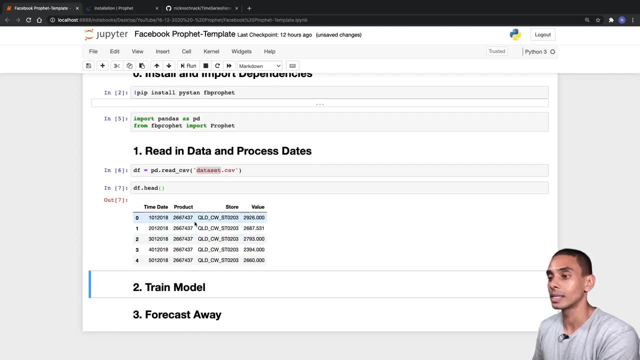 a look at our data set by typing in df head, you can see that it looks pretty similar to what we had in our Excel Notebook, And so it should. Now what we can do is we can take a look at some summary statistics. So if we type in df dot describe, 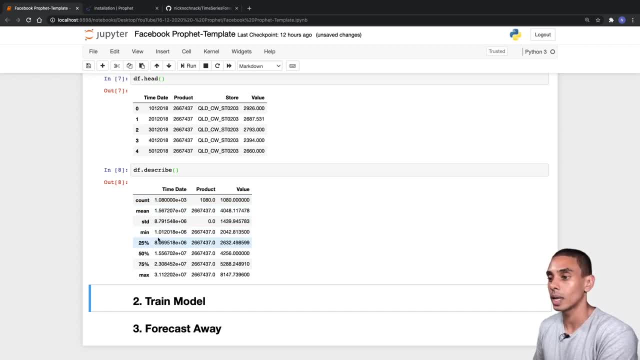 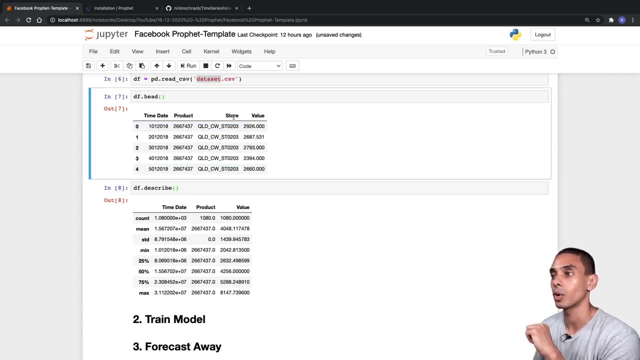 we can see that we've got our count, our mean, our standard deviation, as well as our min and our different quartiles. Now what's most important, though, is we check how many unique values that we've got in product and store, because we want to make sure that we've only got a single value. 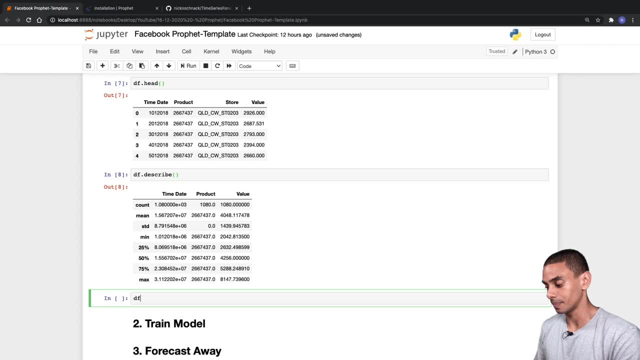 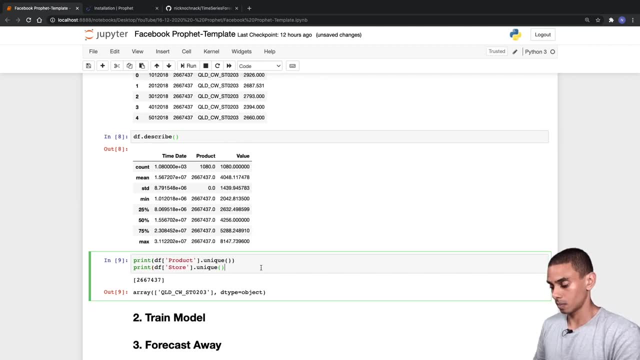 So to do that, we can use the unique method. So let's go on ahead and do that. All righty, so it looks like we've got a single value in both our product and our store column, so it's all good. 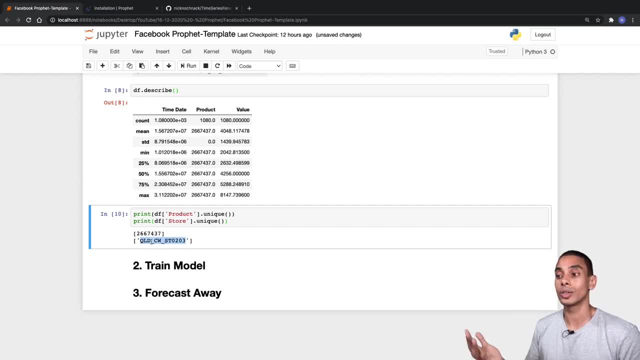 We don't need to do too much additional filtering. What we'll eventually do when we build up our time series forecast, is we're just going to drop these two columns, Because when we actually build a data set for profit, what we actually need is just two columns. So 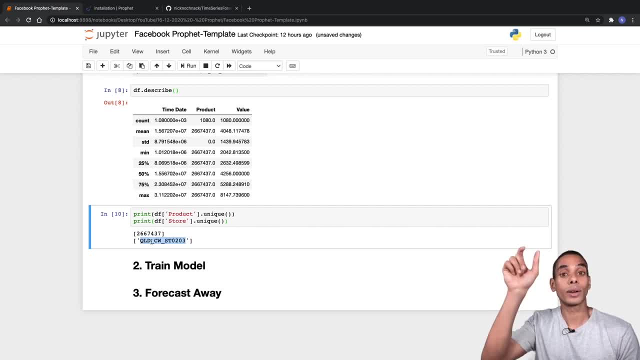 one for ds, which represents our dates, and then one called y, which represents our values. So in this case, our time date is going to represent our dates, after a little bit of pre-processing, and our value is going to be our y column. Now the next thing that we need to do is 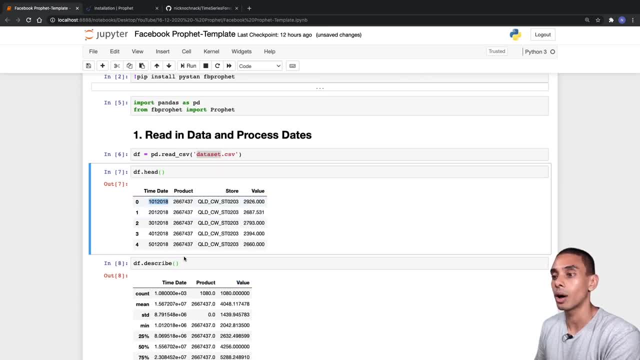 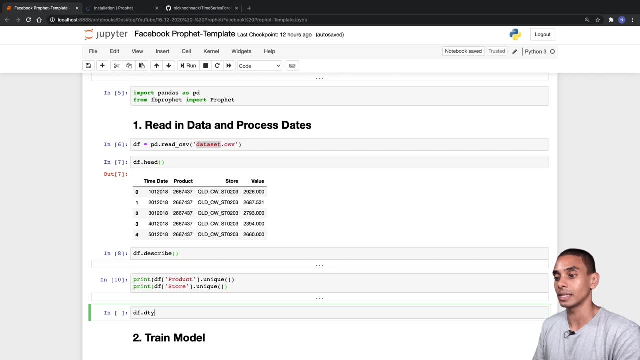 actually process this a little bit, because right now this time date column actually isn't representing our dates appropriately. So if we actually take a look at our data types by typing in dfdtypes, you can see that our time date is just an integer. at the moment. We actually need 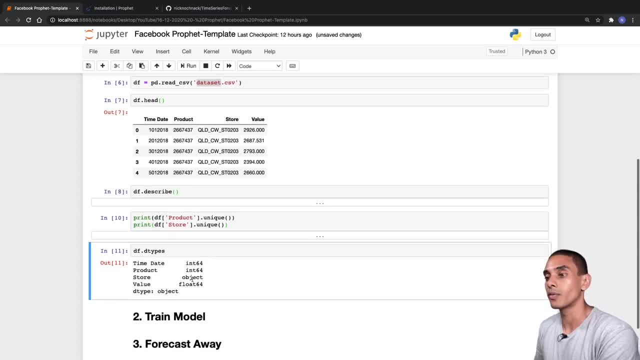 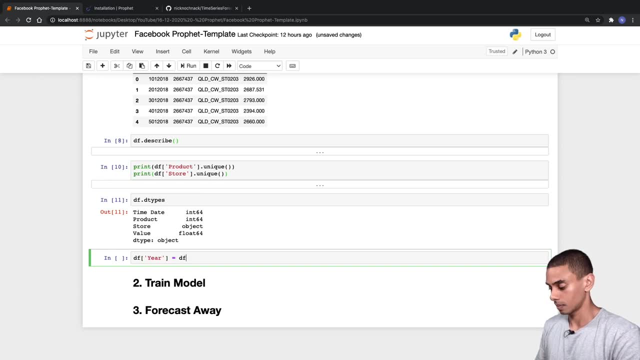 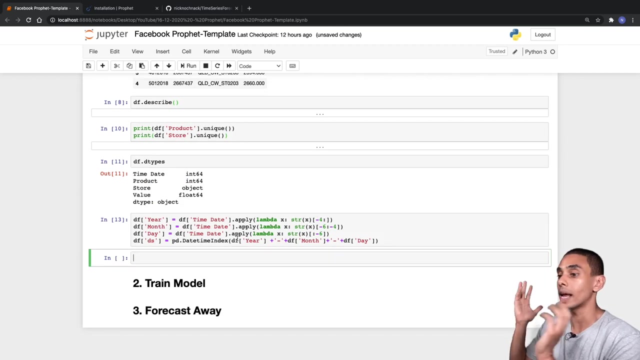 it to be a date time value. So what we're going to do is perform a little bit of pre-processing to convert that into a date time format. So let's go on ahead and start doing that. Alrighty, so we've now gone and done our date pre-processing, So we've written four lines of 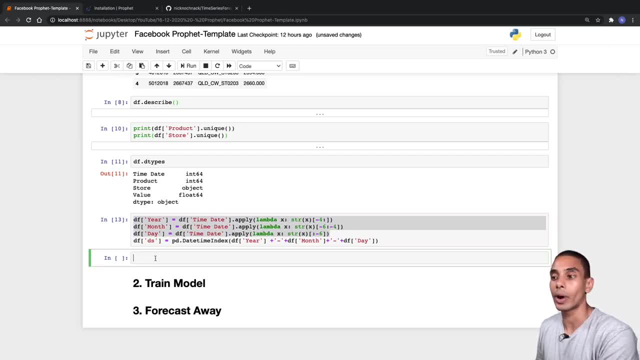 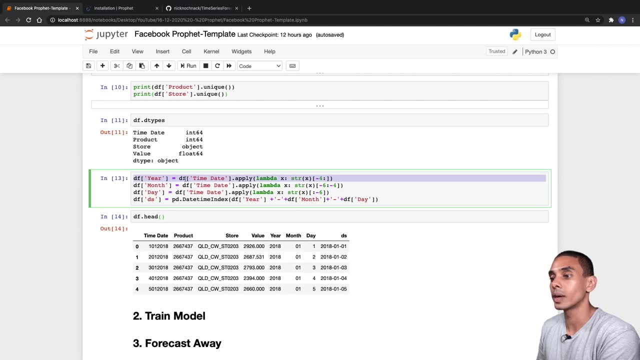 code there. Now, three of these lines are really to do with extracting our year, month and our day. So if we take a look at our top five rows again, so what we're basically doing is we're grabbing our date time column here, so this column, and then we're going through and we're looping through. 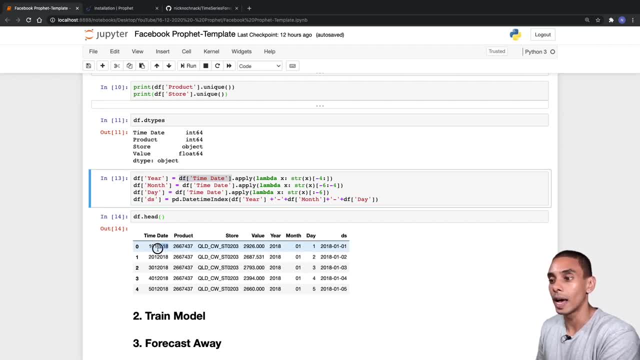 each one of our values and we're grabbing the last four values because this represents our year. So to do that, we've used our lambda function, we've converted our value to our string and then we've gone and grabbed our last four values. So this is just. 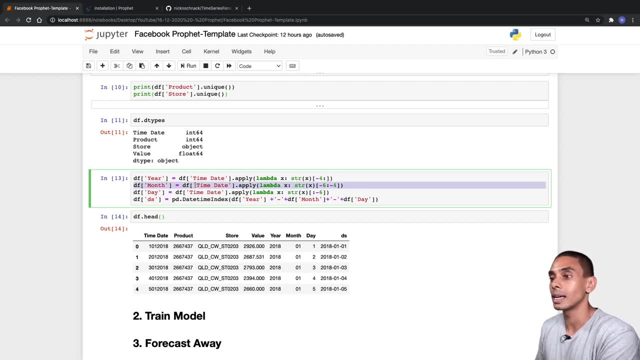 an array indexing method, Then what we've gone and done is done a similar thing for our month and for our day. So in this case our indexing filter is a little bit different. So in this case, to grab our month, we've gone from our sixth value, which will be over here, and we've gone. 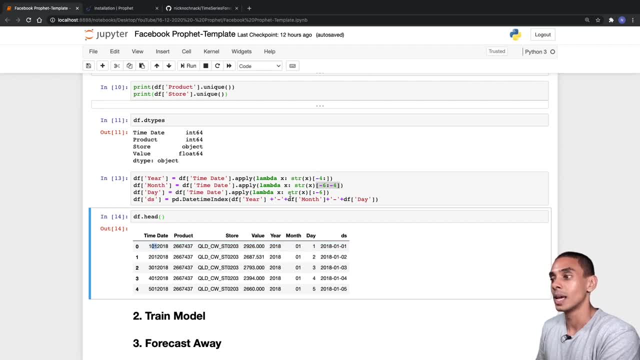 all the way to our negative four value, which will be those two values For our day. we've just gone from six and we've gone out that way, So you can see that the colon is pointing in a different position. And then what we've gone and done is we've concatenated all of those together. 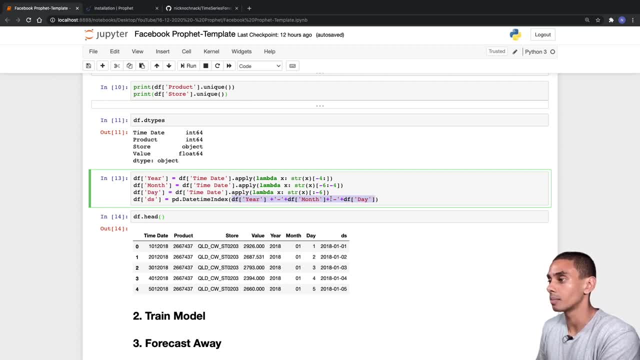 So we've grabbed our year plus and we've added a dash, our month plus, we've added a dash and our day in order to get to this date time value here, And then we've used the pddatetimeindex to convert it to a date time. 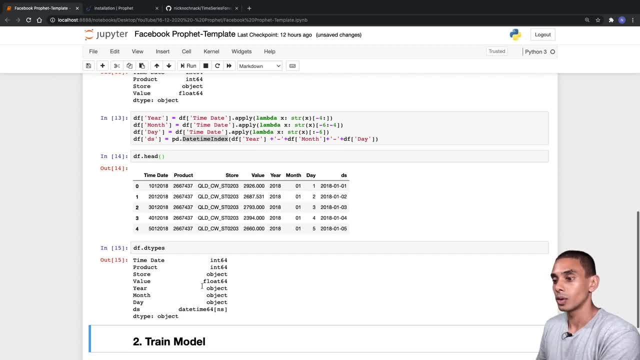 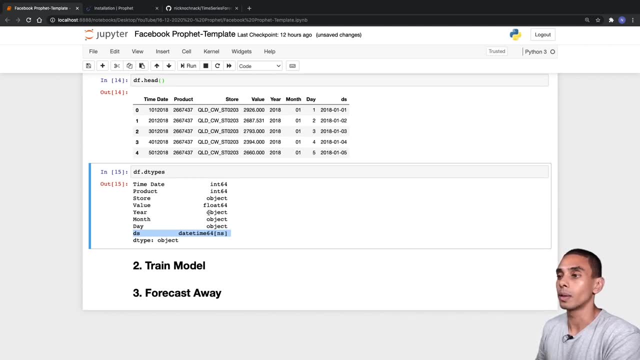 format. So if we actually take a look at our D type now, you can see that our DS column is actually a date time value. So now we're looking good. Now what we can do is drop all the columns that we don't need. So we've got our value column, which we'll eventually rename to y. we can drop our. 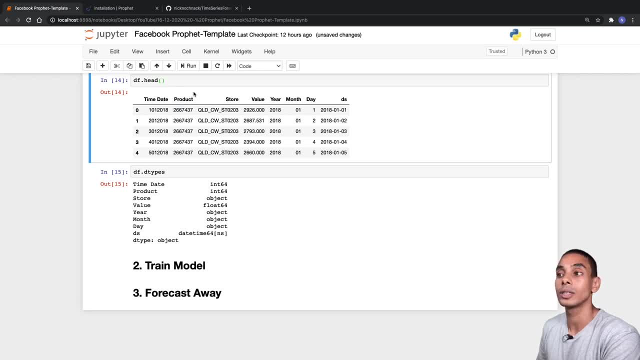 date time column, our product column, store column, and remember we can only drop product and store because they're unique values. So we've only got one product and one store, So we don't actually need these, not adding value. And then we're going to drop a year, a month and a date, So let's go ahead and drop those. 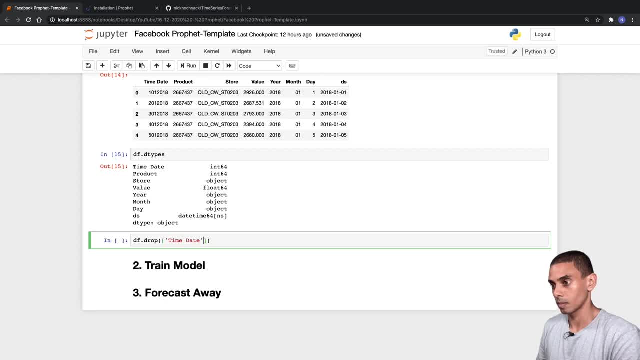 and then we'll rename our columns. Okay, so we've now gone and dropped our column, So to do that we've used different columns, so to use a strong column just to make it more dynamic. But now we're going to add another column and, to bring this down further, we're going to add the volume to the column column. And then we're going to add one column. So we've now gone and dropped our columns. so to do that, we've used the pddattimeindex and we've added a dash our day in order to get to this date time value here. 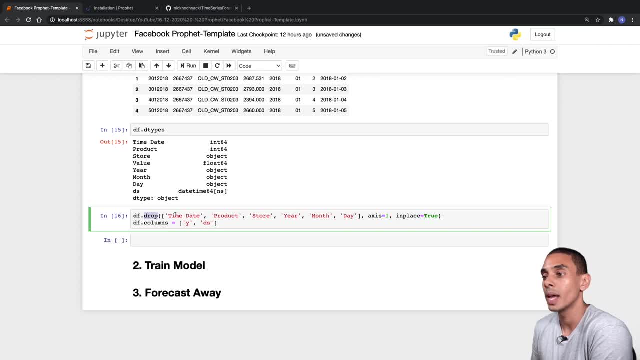 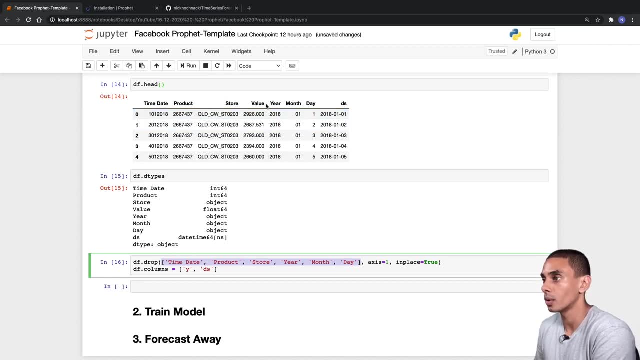 columns. so to do that, we've used the pandas method- drop- and then we've passed through all the columns that we want to drop. so in this case, we want to drop time, date: time date, product, product store, store, year, month, day. so we've dropped all- what is that? six columns- and then we've passed through a. 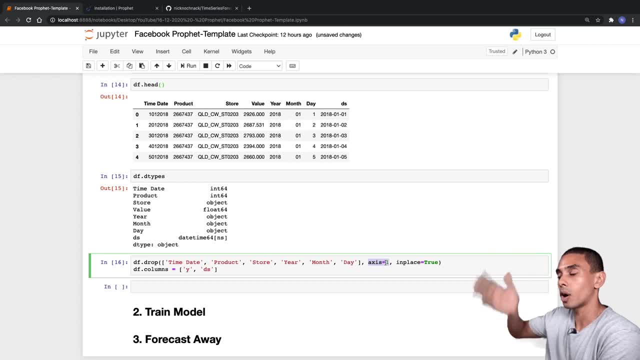 couple of parameters, so we need to pass through access equals one if we're dropping columns rather than rows and then we've specified in place equals true because we want to apply it on that data set, not create a new one, and then what we've gone and done is we've renamed our column. so in this case, 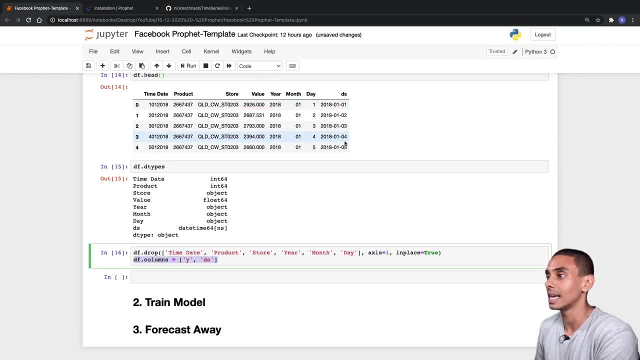 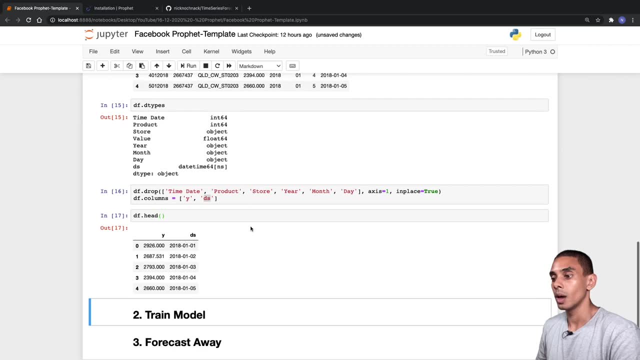 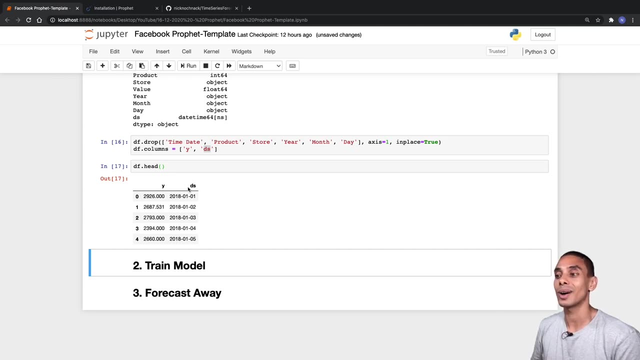 we had two columns left. we had our value and we had our ds column. so we've just renamed them y and then we've left our other column, ds. so if we take a look now, we've now got two columns. and remember i said right at the start, we need two columns in order to work with profit, so we need a y column. 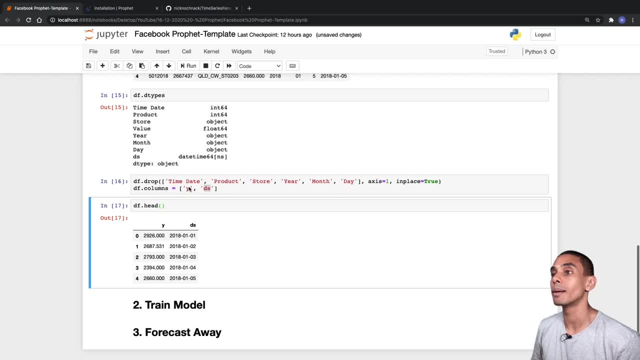 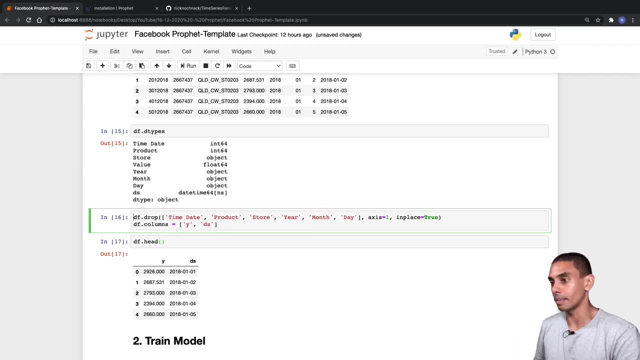 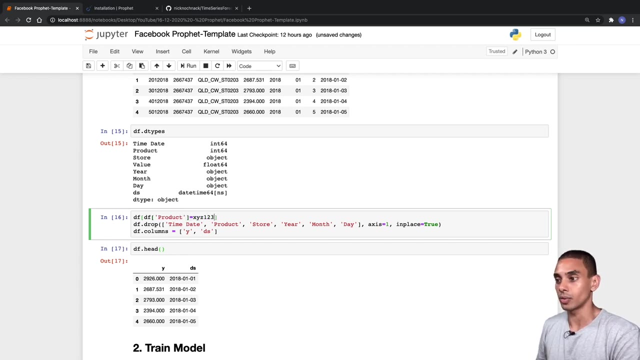 and a ds column. so now we've got them. now if you had multiple products or if you had multiple sets of time series, you can also filter through. so what you can basically do is use a filtering method to filter through. so, for example, we could type in df product equals product xyz 123 and actually make that filter appropriate. so this: 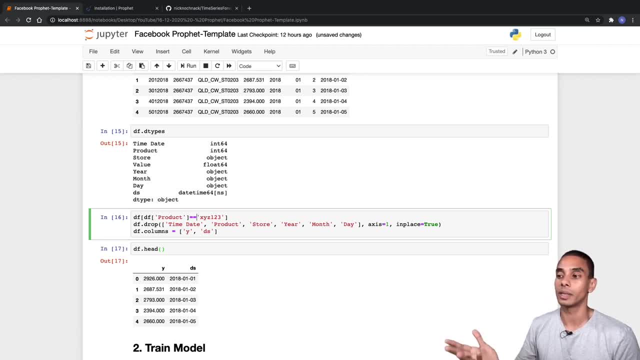 would allow you to filter through and get the specific products or the specific stores or the specific time series that you need. now, in our particular case, we've only got one product and one store, so we don't actually need to do that. but if you came across that, that's how you'd handle. 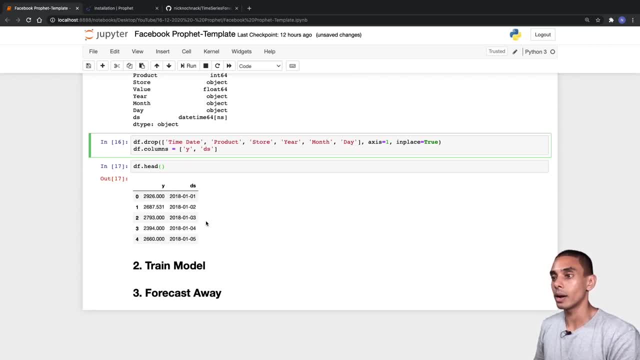 that all righty cool. so we've now got our data set sort of ready for modeling, so let's start building our model. so in this particular case, it's really straightforward. so we just need to instantiate our profit model and then fit it. so let's start doing that. 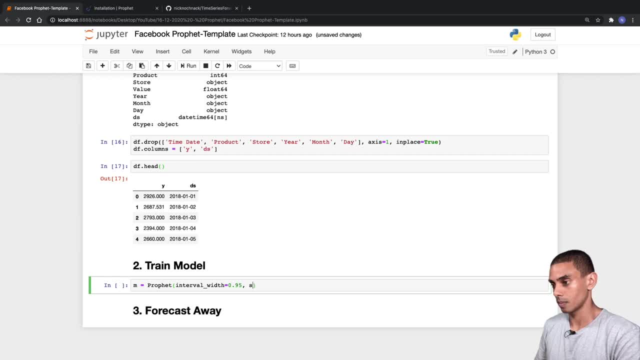 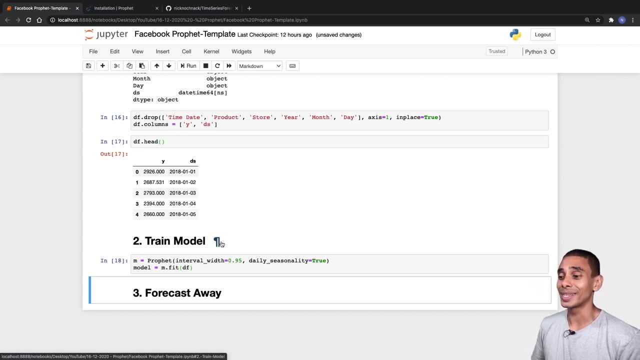 all righty, and that is our model train, so you can see that it trains really, really quickly. that's one of the cool things about profit and one of the things i love about it. it trains really, really quickly and you tend to get quite an accurate forecast. 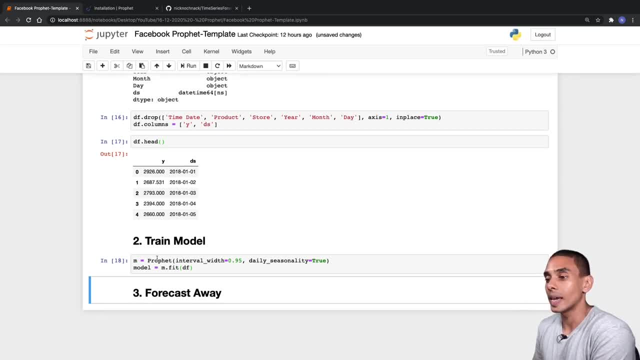 so, in order to train our model, we've written two lines of code, so we've instantiated our profit model. so this is basically saying we're creating a new model, and so to do that, what we've done is we've used our profit class, which we brought in right up here in our install and import step. 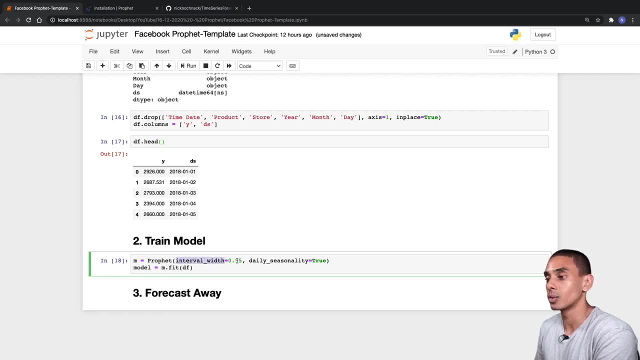 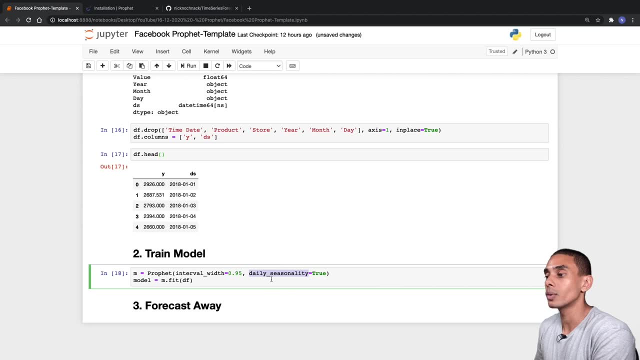 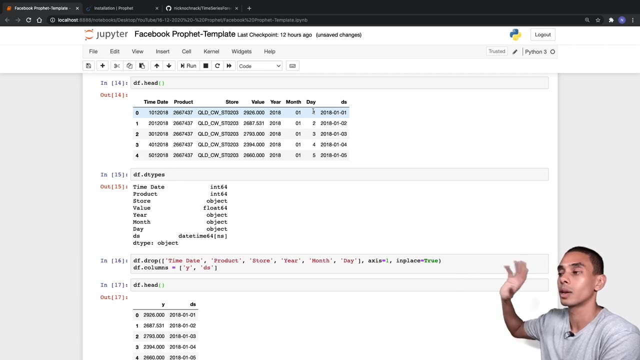 and then we've specified two keyword parameters. interval width equals 95. so this looks at our confidence interval, and then we specify: daily seasonality equals true. now, the only reason we specified daily seasonality equals true is that because we've actually got weights in there, and now I know from previous analysis that we've got a little bit of seasonality. 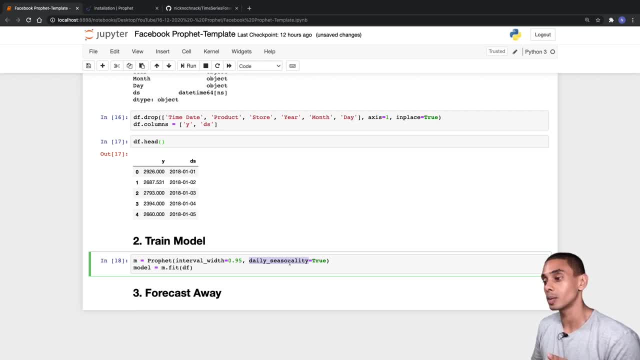 in our days. so we've specified that. but keep in mind, you don't need to specify this. you can actually drop it and you'll still have a model built. then what we've done is we've gone and trained our model. so to do that, we've grabbed our model that we set up up here as variable M and 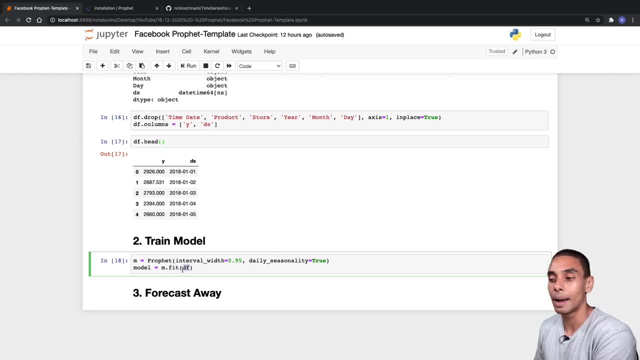 we've used our fit method on our data frame to go and fit our model, so we've now actually got a trained model here. so just by using mfit and then passing through our data frame, we've now got a fit model pretty easy. right now, the next thing that we can do is actually go on ahead and make some predictions. so let's go on ahead and do that. 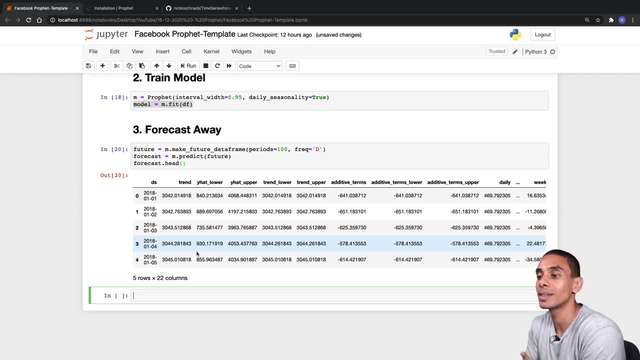 and there you go. so we've now gone and forecasted forward and actually made some predictions. so you can see here that we've now got our data frame. so we've actually got it stored inside of a new data frame called forecast. so from here, whenever you're going and forecasting forward, you're going to get a whole bunch of 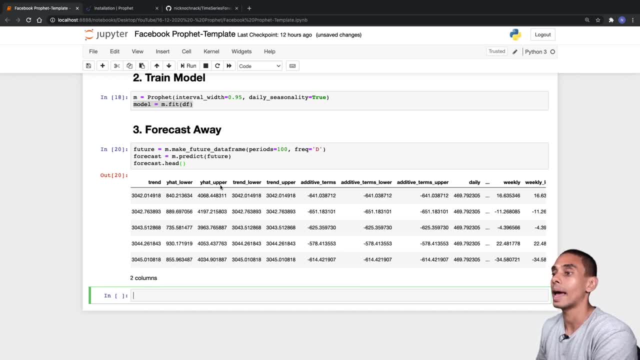 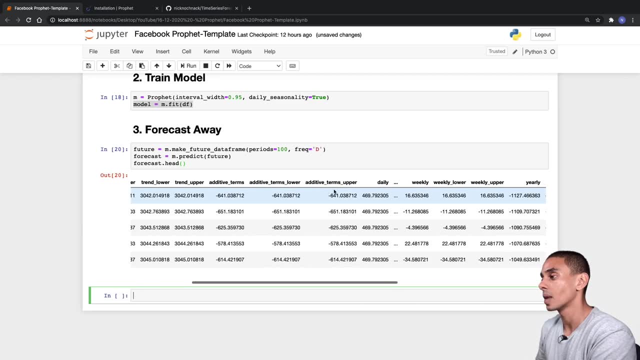 information. so you're going to get your trend, your y hat lower, y hat upper. so these are your upper and lower estimates. you're also going to get your trend, your additive terms, lower and upper. you're also going to get your daily seasonality, so on and so forth. now, if you scroll all the way to the right, 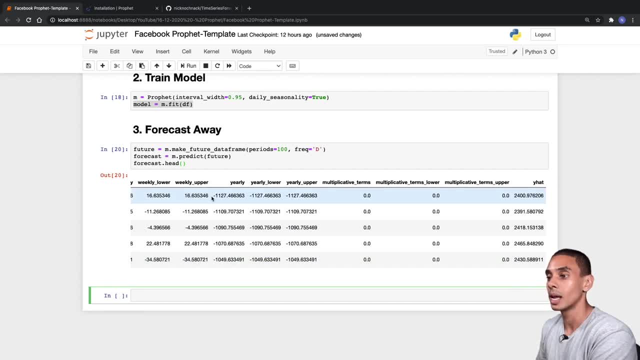 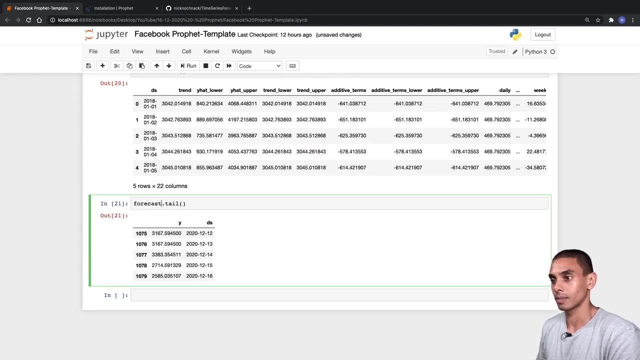 you're going to get this column y hat and that represents your prediction now. right now, we're taking a look at the top row, so this isn't actually our future periods, but if we'd look at the bottom, so if we look at the tail set of our forecast data frame, you can see that we've 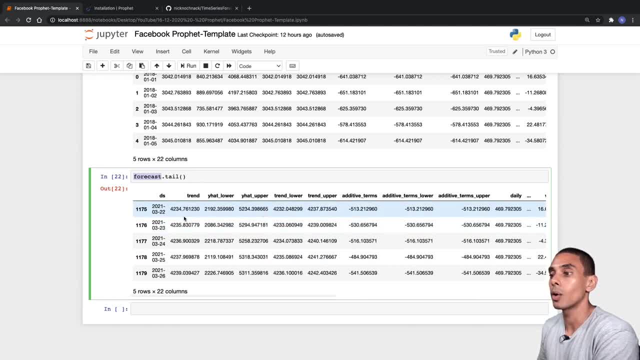 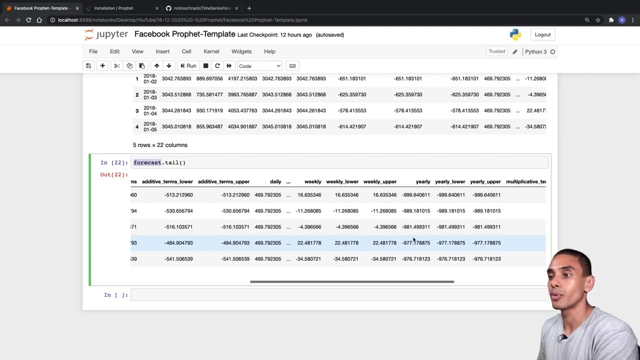 got our future forecast periods forecasted out. and again, you've got all of this additional information, so it gives you more than just a straight forecast. you get a whole heap of additional terms, the trend y hat upper, lower. you get your additive terms, what your weekly trends and what your weekly effects look like, so you can actually break this out into a really 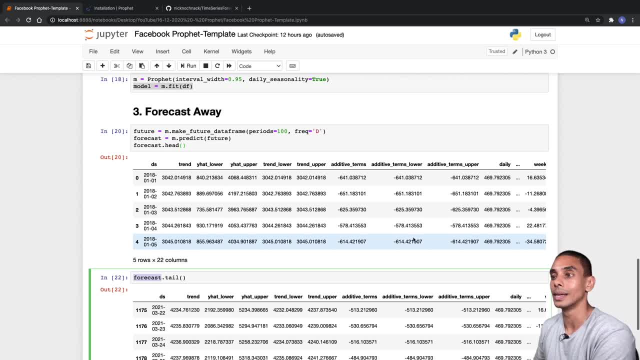 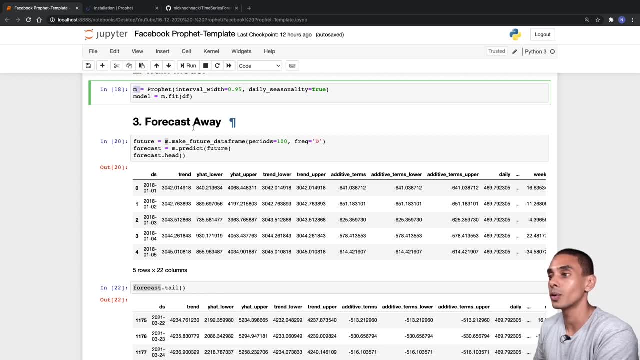 really detailed time series forecast. now let's take a look at how we actually did this. so, again, using our trained model, what we did, so remember, we set up our variable M, which held our profit model. we ran the make future data frame method, and to that we pass through the number. 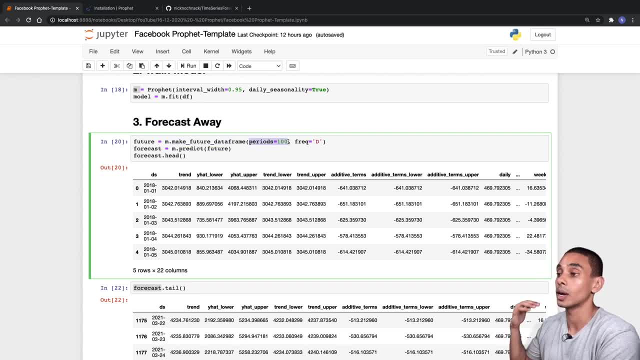 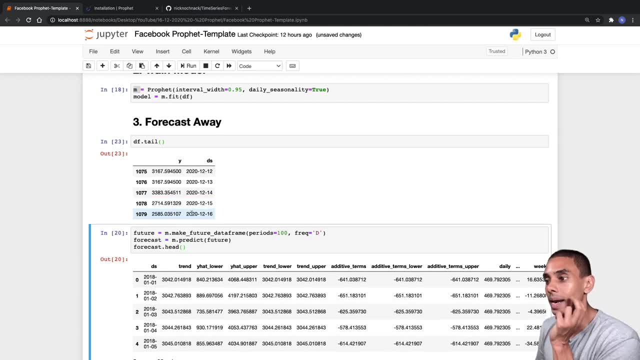 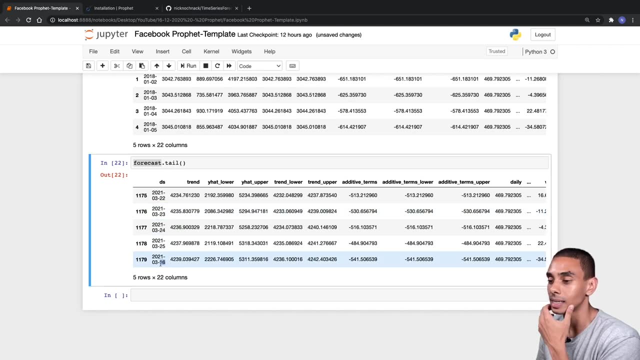 of periods that we want to fall forecast forward. so we forecasted periods up to 100. so if we take a look at the tail of our data frame, or our main data frame, you can see that we went up to about the 16th of December 2020.. now, from our forecast that goes all the way out to the 26th of March. 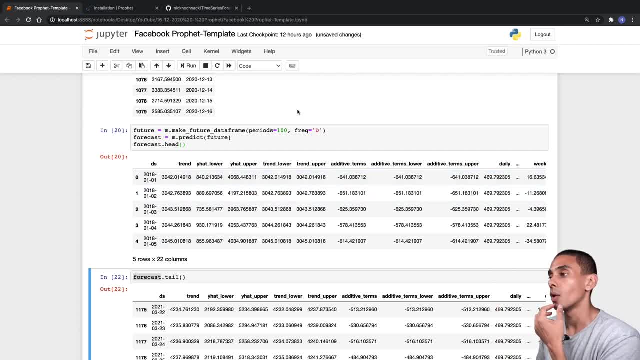 2021, so it actually pushes further forward. so we then specified our frequency: so we want it by day. and then what we did is we use the predict function and we pass through our future data frame, so the one with our additional periods to go on ahead and forecast forward. so again, we used 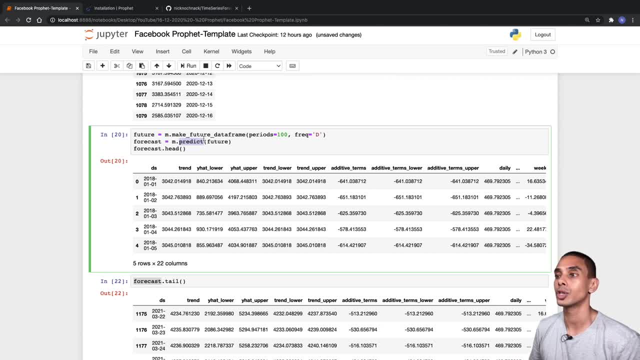 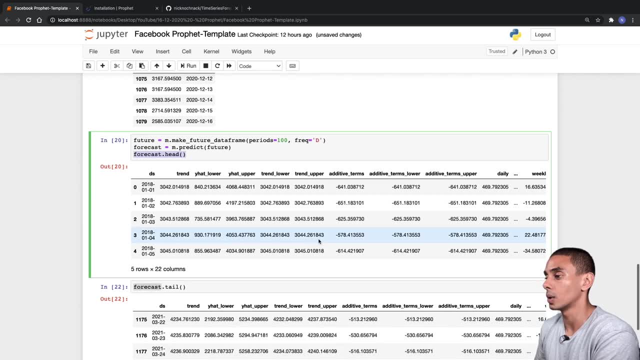 the predict function there. so pretty similar to when you're building different machine learning models: you fit using the fit method and you predict using the predict method. then what we did is we use the head method to display the first five rows, which again is our historical data. but 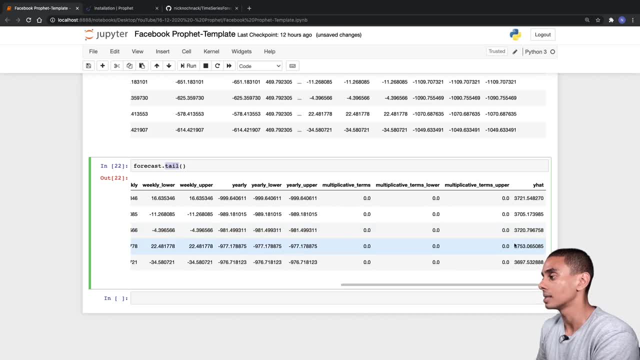 the tail, so, forecasttail, we're going to be able to see our forecast now. if we wanted to just extract our dates and our actual prediction, we can just do a quick filtering method and that's going to give us just our two columns that we want. so you can see now that we've only 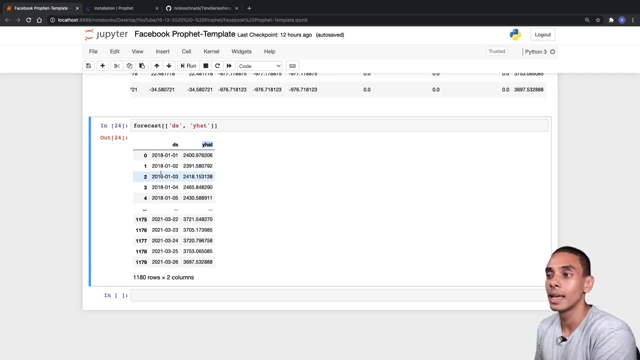 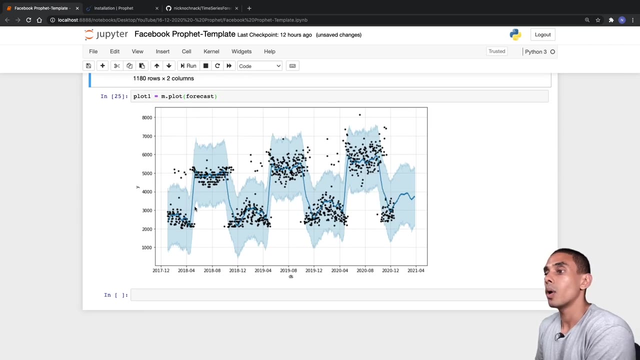 got our date and our predicted forecast. now again, these are going to be our historical periods. these are our future predicted periods, so this gives us quite a fair bit of information as to what our forecast looks like now. if we want, we can plot these out, and so what you're basically getting here is: the blue line represents your prediction, or 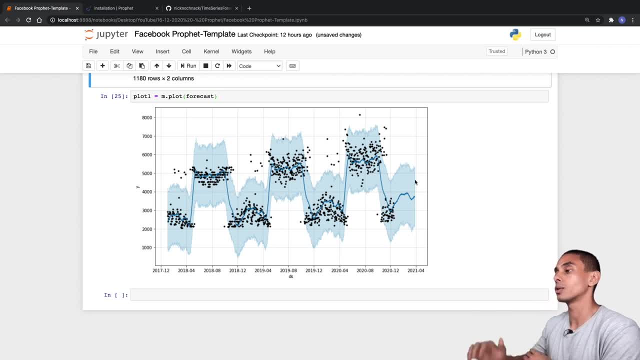 your y-hat value. these shaded blue regions represent your different bounding boxes. so your y-hat upper and your y-hat lower. so you can see that our data set has a little bit of seasonality during the earlier months and then spikes up, goes down, goes up, then goes back down. 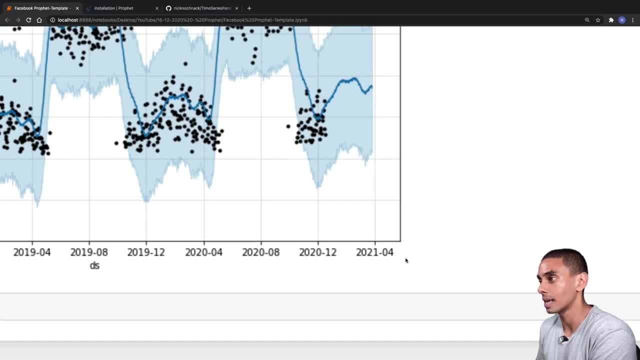 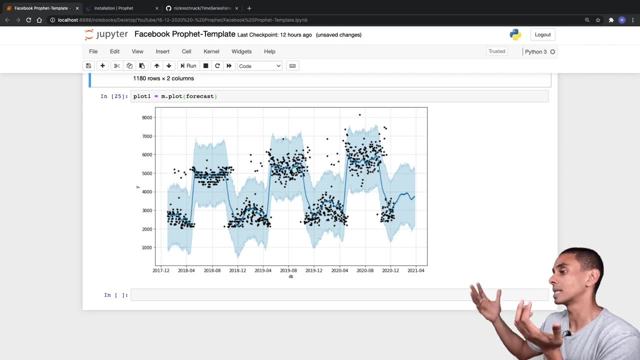 and goes up and you can see that in our forecast period. so we've got them down here, that we are in making that pattern. so you can see that we're pretty close to estimating within a range what our predicted periods look like. so our black dots are our actual values from our forecast blue line. 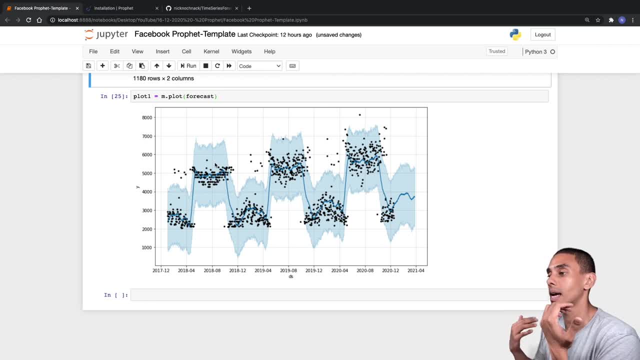 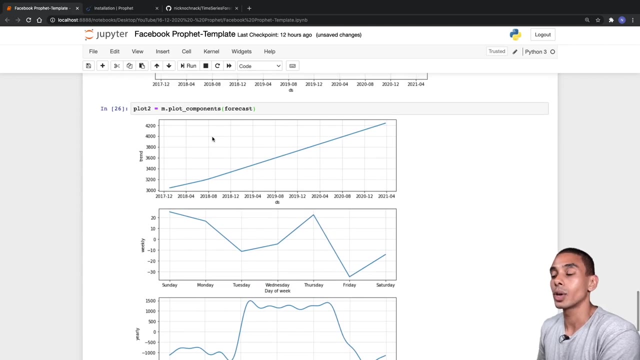 is our prediction, or our y-hat, and our shaded area represents our different bounding boxes. now, one of the other cool plots that you actually get inside a profit is the ability to decompose your trend. so let's take a look at that and there you go. so to do that what we've done. oh, we didn't actually explain. 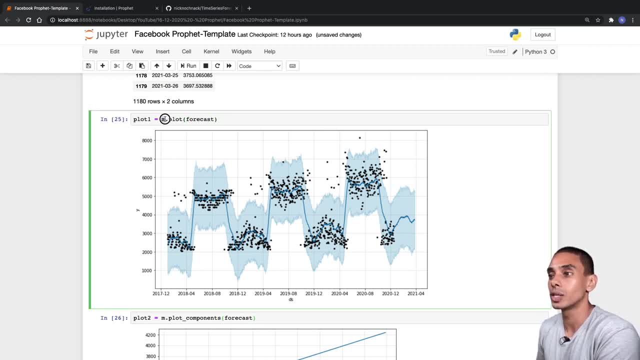 the last bit. so in order to get this chart up here, all you need to do is grab your profit models. in this case it's stored in variable M, as we took a look at before, and then we just ran the plot method then to that we pass through our forecast data frame, which we had from our prediction over here. 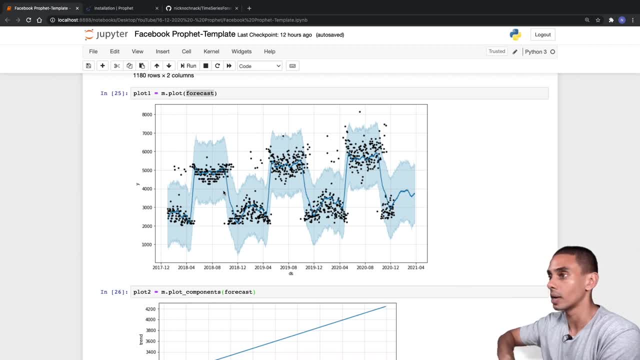 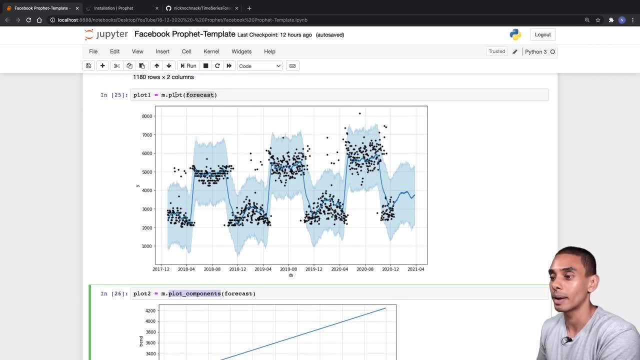 and that gives us our plot automatically. so these are built into profit, so you don't need to do anything additional, it just sort of comes up. then the next plot that we've done is we've plot our component so up here. we just did a straight plot. here we again. 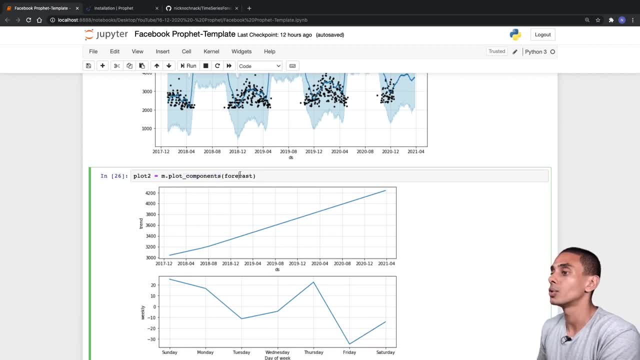 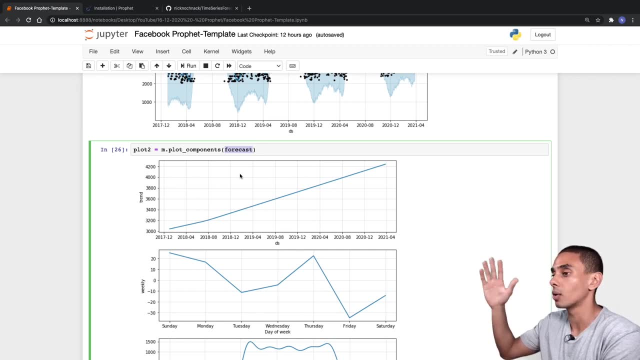 grabbed our profit model and we use the method plot components to that. we pass our forecast data frame. now this gives you a lot of information about your different Trends, whether or not it's all weekly or daily seasonality. so it's nice to know that it's breaking down and decomposing your 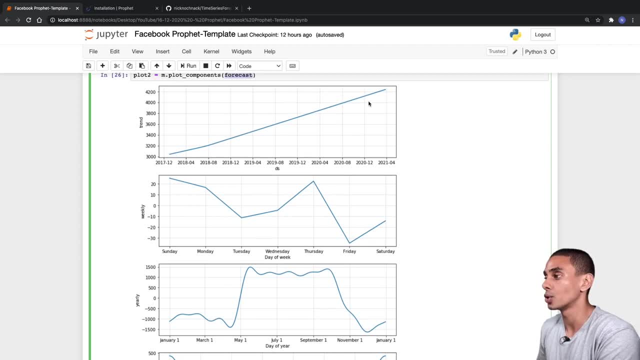 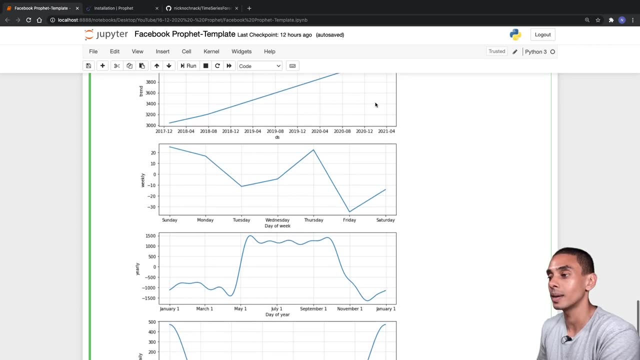 data set, so you can see here that our overall trend is pushing upwards, and so this basically is stating that from 2017 to 2020-ish, we were looking at an upward Trend. we can also take a look at our weekly Trend, so it looks like we may be sold a lot more. 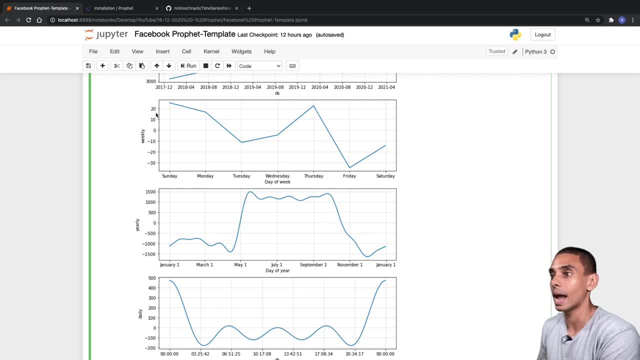 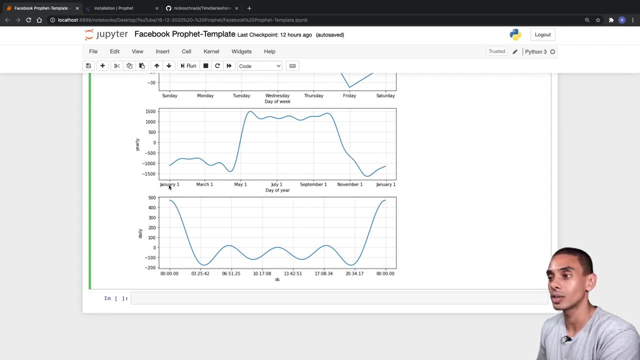 on Thursday, sold a lot less on Sunday and we sort of averaged out on the other days and if we take a look at our yearly seasonality, so you can see that over our earlier months- so January to what would that be April-ish- we're selling less. likewise in our later months of Jan or our earlier months of. 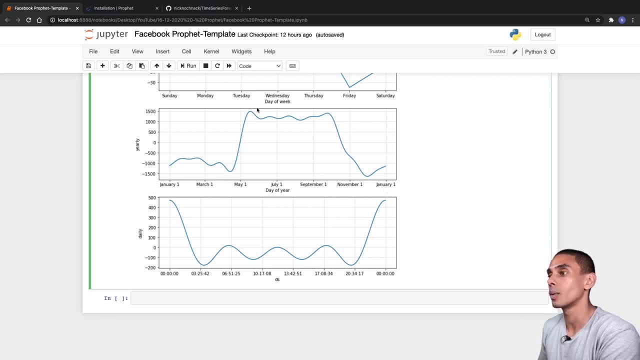 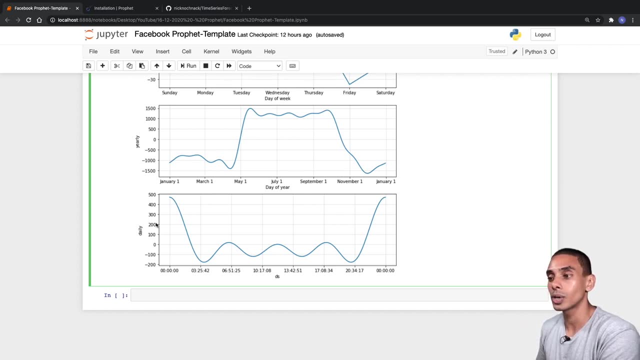 Jan, whichever way you want to take a look at it. and then during the middle of the year, we're selling a lot more, so maybe there's- this could potentially be something to do with the weather or seasonality in that respect- and then we've also got daily seasonality. 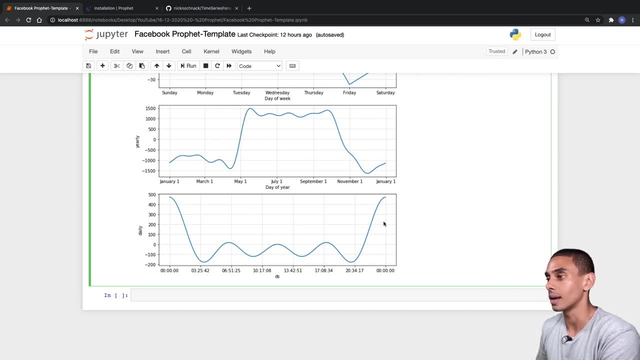 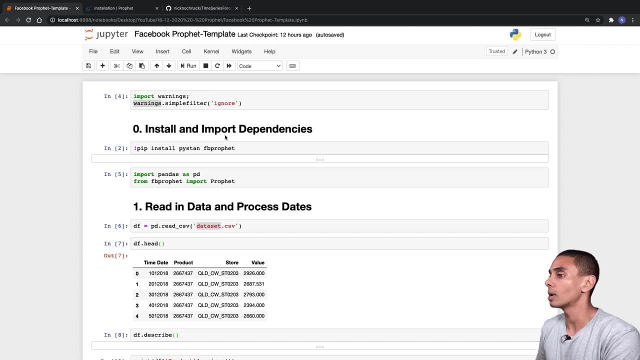 as well, and this actually takes a look at how the day and the time affects our sales. and that about wraps it up. so that's how to build a forecast using the Facebook profit package. so we've done quite a fair bit. so we installed our libraries. so, using pip, install pi, standard Facebook profit. we then 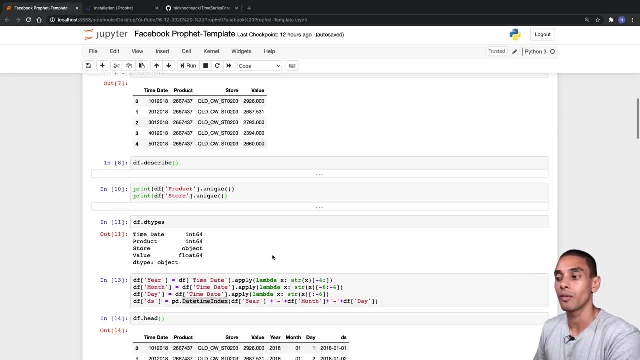 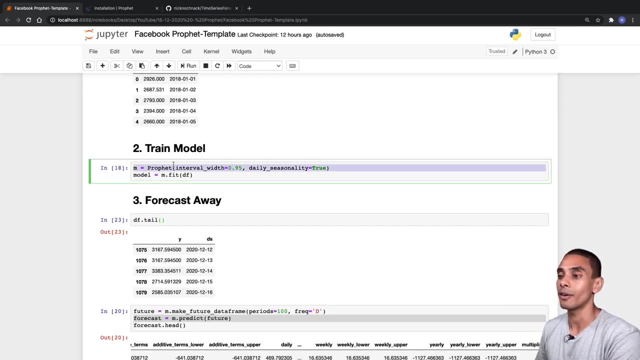 read in our data set using the pdread CSV method and performed a bunch of date transformations. then we went and trained our models. so again, pretty easily just two methods. so mprofit or m equals profit, and then mfit to fit. and then we went and 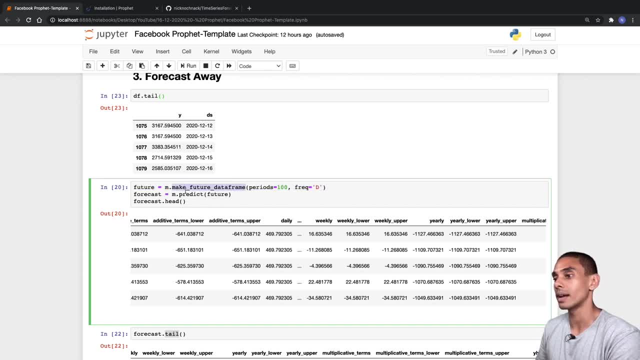 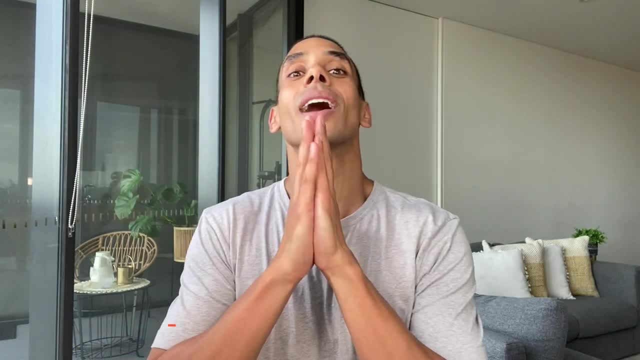 forecasted our model. so these two key lines here so make future data frame and mdot predict, allow you to go and build your forecast. and that about wraps it up. thanks so much for tuning in, guys. hopefully you found this video useful. if you did, be sure to give it a thumbs up, hit, subscribe and.